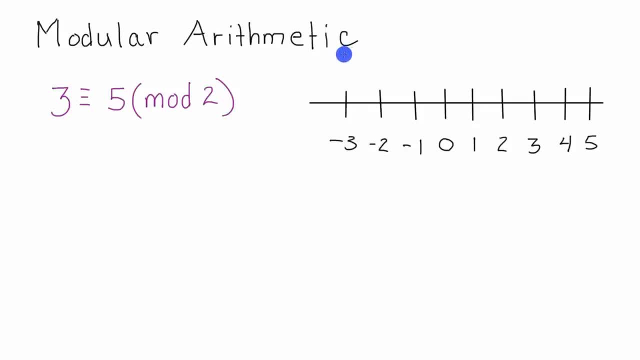 Modular arithmetic is a very fundamental component of cryptography, so it's very important that we understand what modular arithmetic is and how to use it before we ever start learning about cryptography. 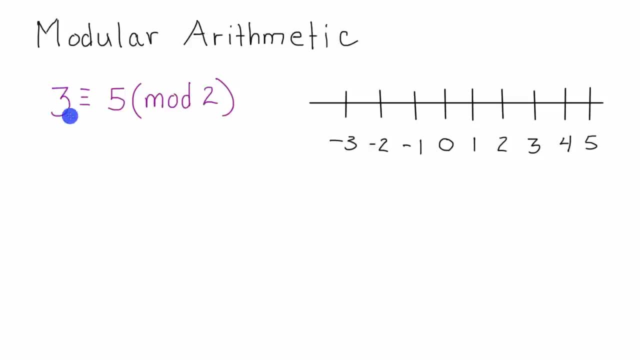 Here I have a statement, and what the statement says is it says 3 is congruent to 5 mod 2. So essentially what that's saying is in the world of mod 2, 3 and 5 are equivalently the same thing. So how exactly does that work? Well, let's look at this number line right here. We'll go ahead and place 3 on this number line. So there's a 3, and now we'll go ahead and place 5. And so now we have the numbers 3 and 5 on our number line. But 3 and 5 are 2 distinct. However, we're dealing with mod 2 in this case. So the 2 here in mod 2 tells us how many values we can have in mod 2. That means there's only 2 values in mod 2. So for every mod, the value starts at 0, and it ends at one number less than the mod. So one number less than 2 is 1. So for mod 2, the acceptable values are 0 and 1. If we were dealing with mod 3, we would have 3 values to work with, starting at 0, then 1, and going forward. 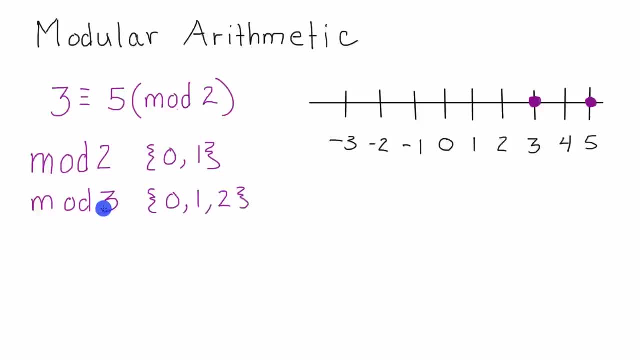 So mod 1 is going up to 2. 0, 1, and 2. 3 values in mod 3. 0 and 1 gives us 2 values for mod 2. If we wanted to take this further, we could take a look at mod 9, and the acceptable values for mod 9 would be 0 all the way up to 8, giving us 9 numbers. So I think you guys can see the pattern here. The mod number tells us how many values we have in our mod, and the highest number of the mod is always 1 less than the mod itself. 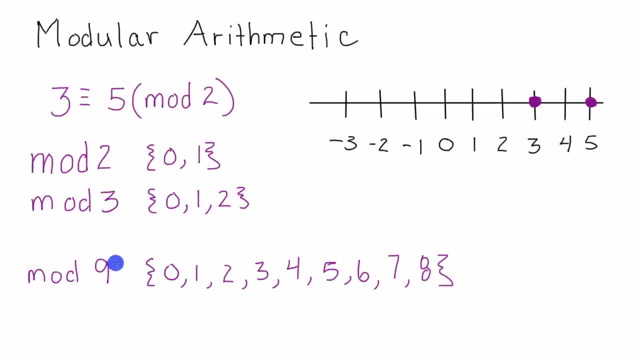 So 3 goes up to 2. 2 goes up to 1. 9 goes up to 2. up to eight. So how do we apply these values to our number line here? Well we start at the zero 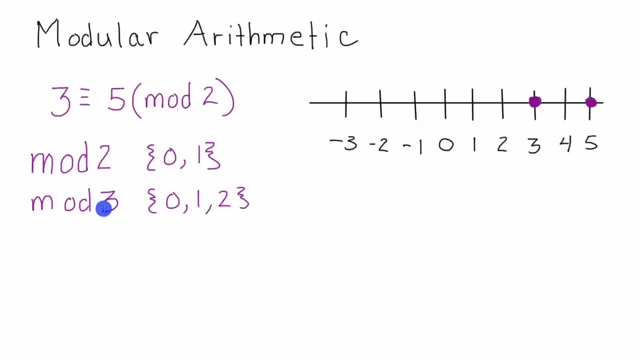 And so mod 3,, 0,, 1, and 2.. So 3 values in mod 3.. 0 and 1 gives us 2 values for mod 2.. If we wanted to take this further, we could take a look at mod 9, and the acceptable values for mod 9 would be 0 all the way up to 8, giving us 9 numbers. 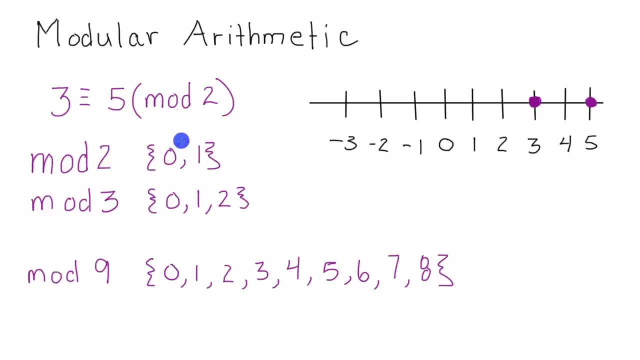 So I think you guys can see the pattern here. The mod number tells us how many values we have in our mod, and the highest number of the mod is always 1 less than the mod itself. So 3 goes up to 2,, 2 goes up to 1,, 9 goes up to 1.. 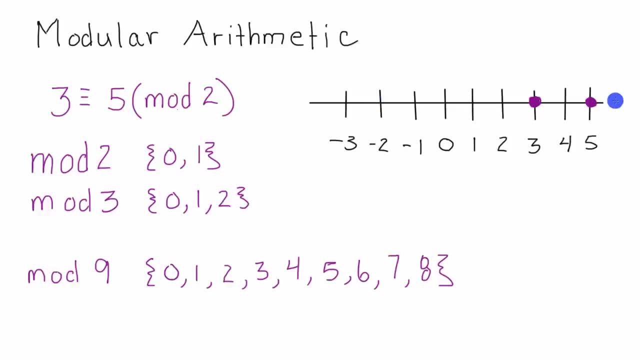 up to eight. So how do we apply these values to our number line here? Well, we start at the zero, and for the moment we'll look at mod two. So the possible values we can have for mod two are the numbers zero and one. So we start at zero and then the next number would be one. So then we would 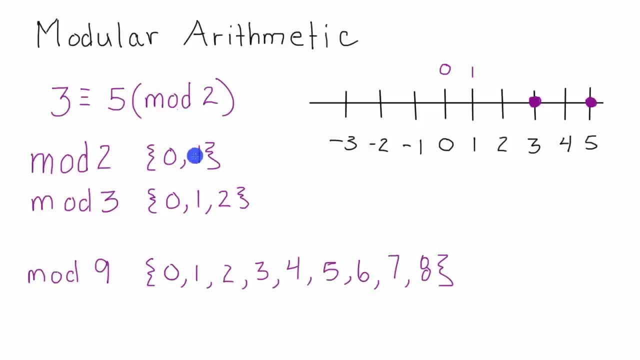 want to put a two, but two isn't one of the acceptable values, So we switch back to the beginning. So this becomes zero one, zero one. So three has the value one in mod two and five also has the value one in mod two as well. So therefore three and five essentially have the same value. 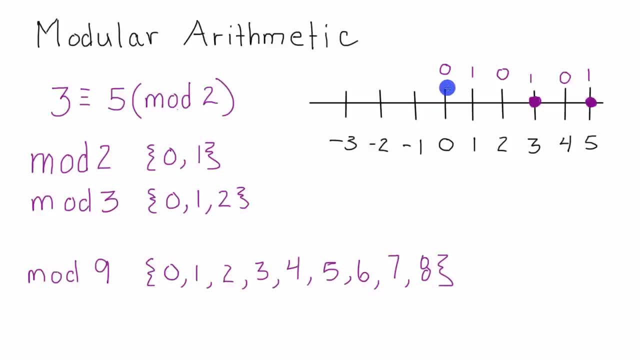 when we're dealing with mod two. We can also apply this to negative numbers as well. So, following this pattern, negative one would have the value of one in mod two, Negative two would have the value of zero in mod two and negative three has the. 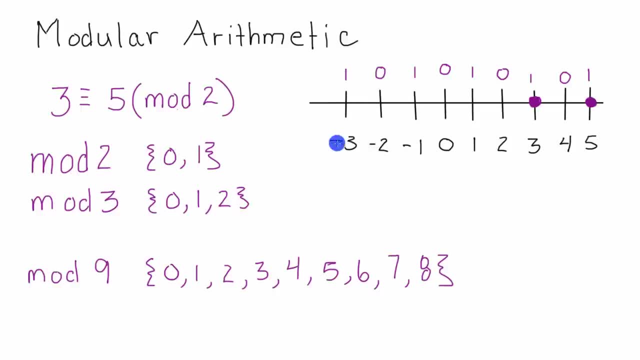 value of one in mod two. So we can apply this to our number line here. So we start at zero and then the next number would have the value of one in mod two. So in mod two negative three is congruent to positive three and negative three is congruent to five, because both negative three. 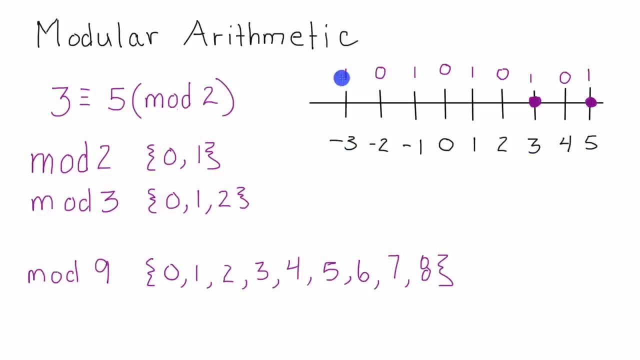 three and five correspond to the number one when we're dealing in mod two. Let's take a look at this with mod three now. So when we want to plot the numbers for mod three, we're going to use the same approach that we used when we plotted the numbers for mod two. So zero always maps to zero. 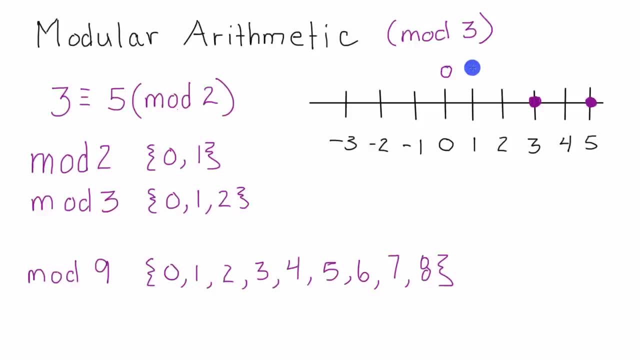 and then we start counting up in mod three. So one is one, and then we start counting up in mod three, So one is one, two is two, and then we would want to do three next. but when we're dealing with mod three, our only possible values are zero, one and two. So since we've already got to two here, we start over. 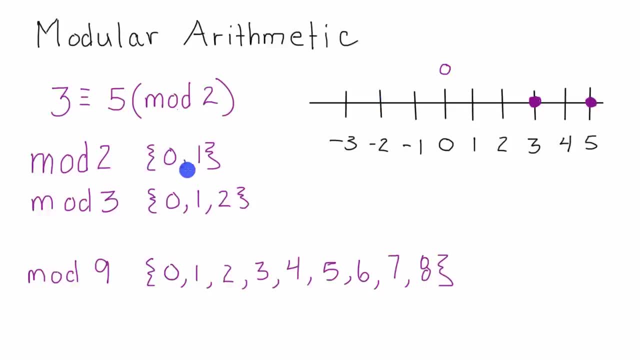 and for the moment we'll look at mod two. So the possible values we can have for mod two are the numbers zero and one. So we start at zero and then the next number would be one. So then we would want to put a two but two isn't one of the acceptable values. So we switch back to the beginning. So this becomes zero one zero one. So three has the value one in mod two and five also has the value one in mod two as well. So therefore three and five essentially have the same value when we're dealing with mod two. We can also apply this to negative numbers as well. So following this pattern negative one would have the value of one in mod two. Negative two would have the value of zero in mod two and negative three has the value of one in mod two. So we can apply this to our number line here. So we start at zero and 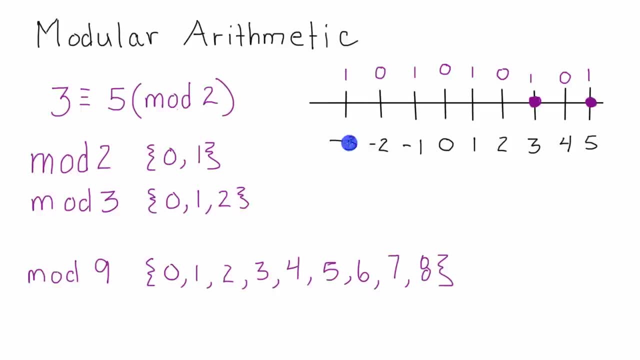 then the next number would have the value of one in mod two. So in mod two negative three is 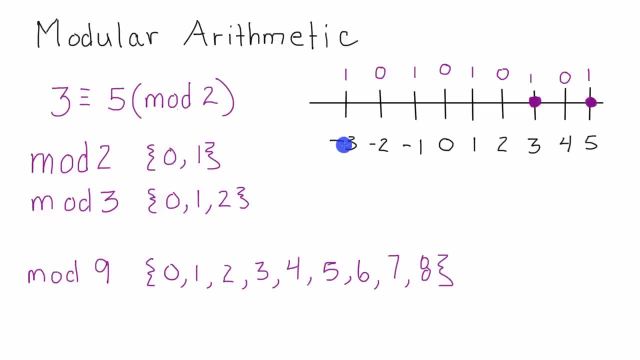 congruent to positive three and negative three is congruent to five because both negative three three and five correspond to the number one when we're dealing in mod two. Let's take a look at 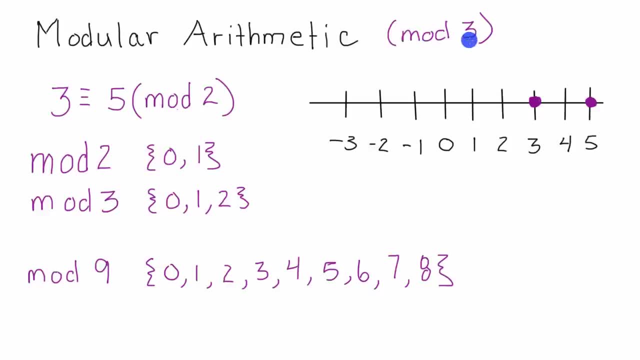 this with mod three now. So when we want to plot the numbers for mod three we're going to use the same approach that we used when we plotted the numbers for mod two. So zero always maps to zero and then we start counting up in mod three. So one is one and then we start counting up in mod three. So one is one two is two and then we would want to do three next but when we're dealing with mod three our only possible values are zero one and two. So since we've already got to two here we start over at zero again. So four becomes one and five becomes two. So we just create this pattern all the way across the number line zero one two zero one two zero one two and it just keeps repeating. So therefore all of the integers on the real number line will map to zero one or two when we're dealing with mod three. We can also use the same approach to plot the numbers for mod three. So we start with the negative direction. So we'll start with the negative and then we'll also take this in the negative direction as well. So going backwards now starting at the other end two one zero. So negative three is congruent to zero in mod three and positive three is congruent to zero in mod 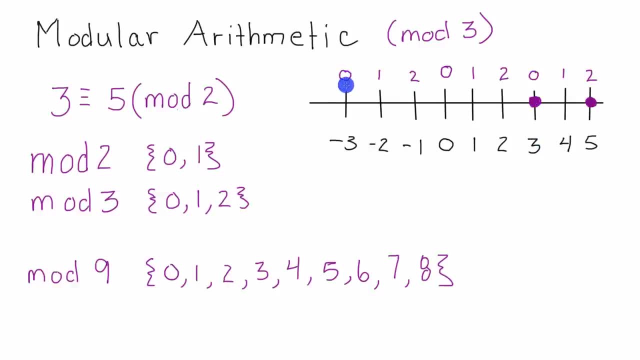 three. Notice how I went backwards here in the negative direction but if we read this left to right again we continue the same pattern zero one two zero one two zero one two and it just keeps repeating. If we're looking at three and five in mod three we're going to start with the negative